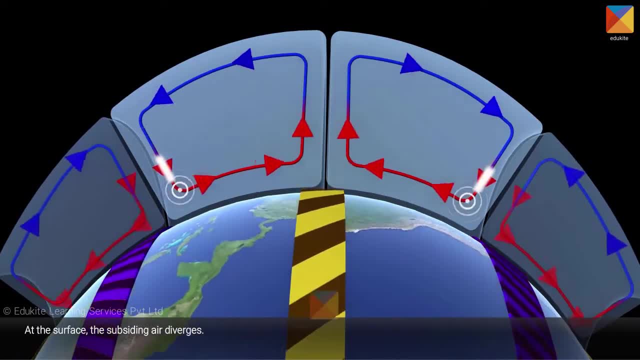 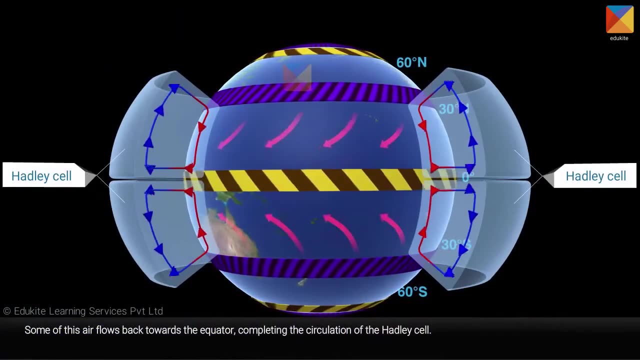 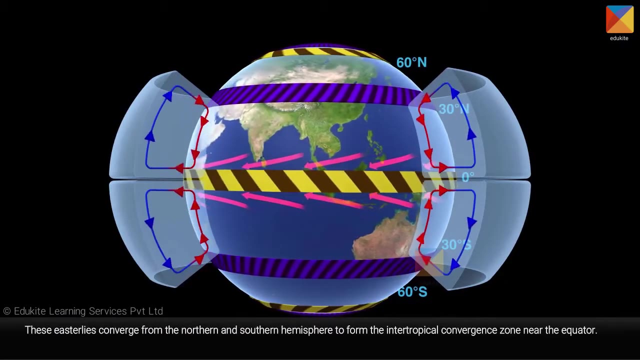 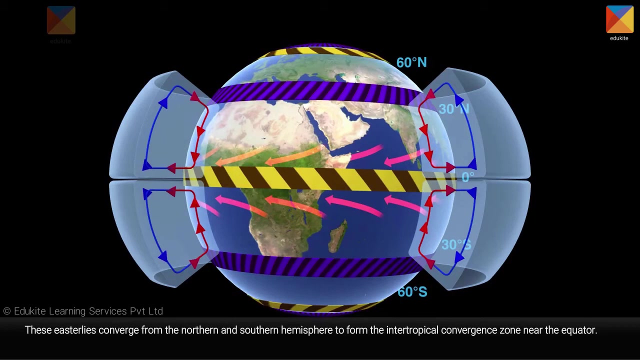 At the surface, the subsiding air diverges. Some of this air flows back towards the equator, completing the circulation of the Hadley cell. This surface flow forms the tropical easterly winds. These easterlies converge. They converge from the northern and southern hemisphere to form the intertropical convergence zone near the equator. 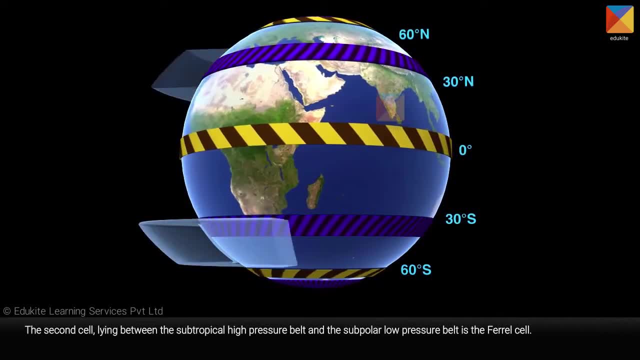 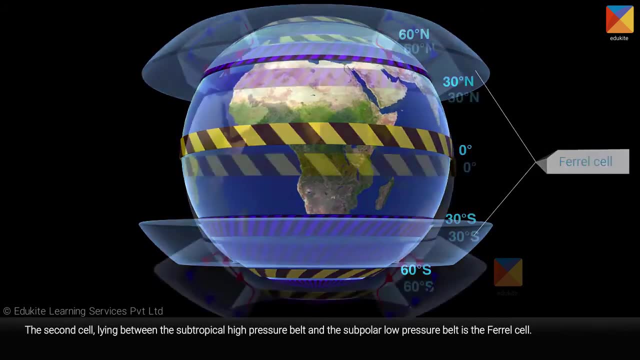 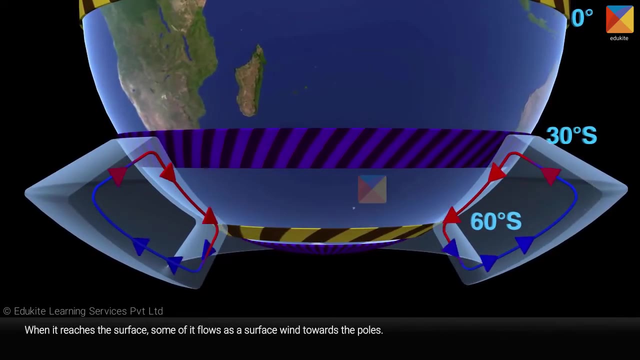 The second cell lying between the subtropical high pressure belt and the subpolar low pressure belt is the Ferrell cell. At 30 degrees north and south, the air warms as it subsides or sinks When it reaches the surface. some of it flows as a surface wind towards it. 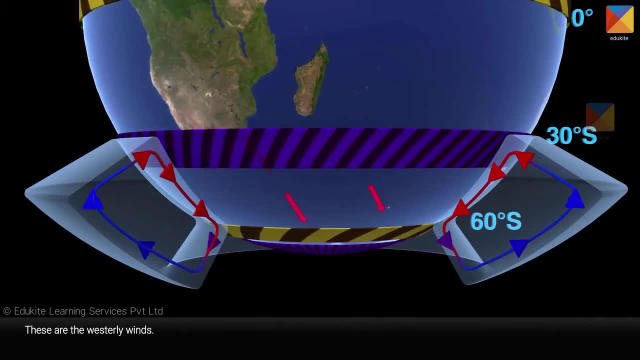 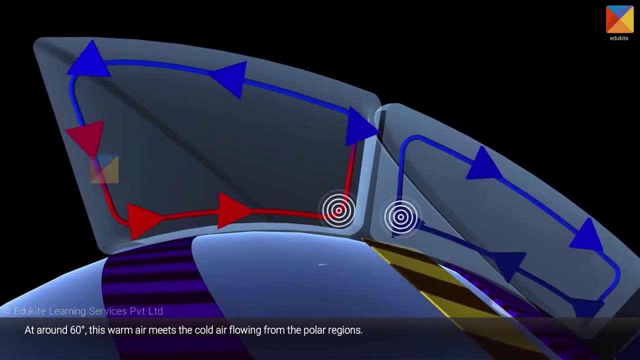 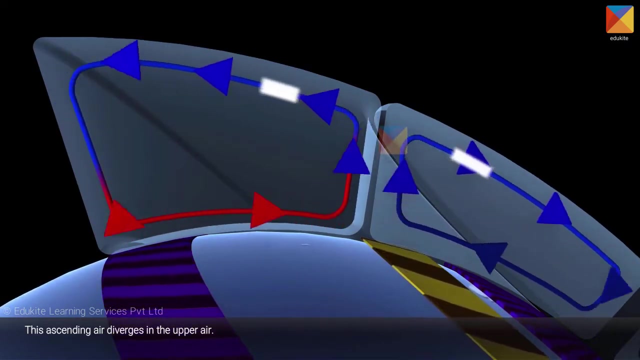 It shifts towards the poles. These are the westerly winds At around 60 degrees. this warm air meets the cold air flowing from the polar regions. This convergence of air causes the air to rise. This ascending air diverges in the upper air. 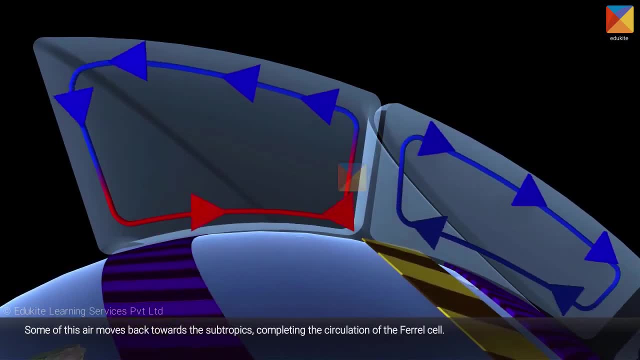 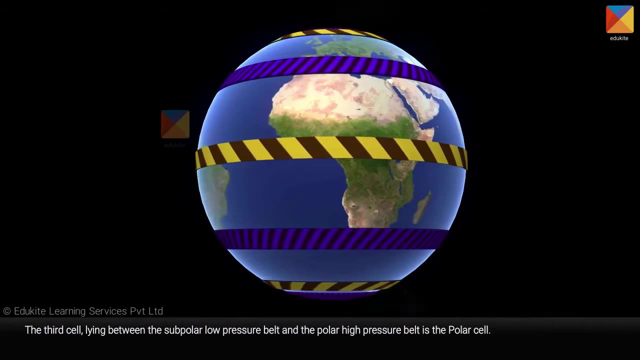 Some of this air moves back towards the subtropics, completing the circulation of the Ferrell cell. The third cell lying between the subpolar low pressure belt and the subpolar low pressure belt is the Hadley cell pressure belt and the polar high pressure belt is the polar cell. 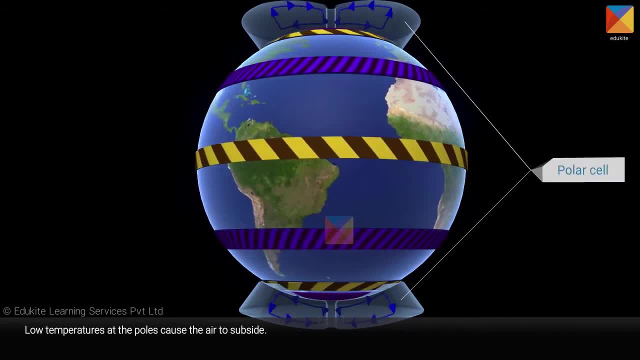 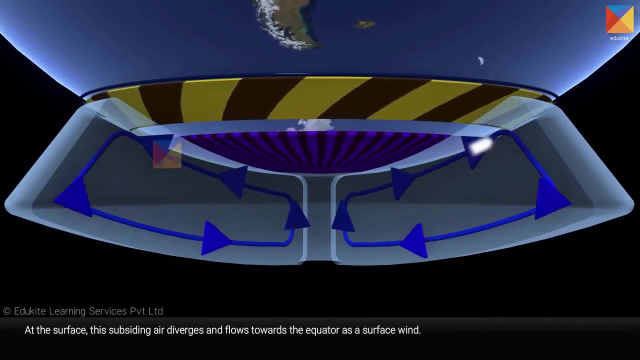 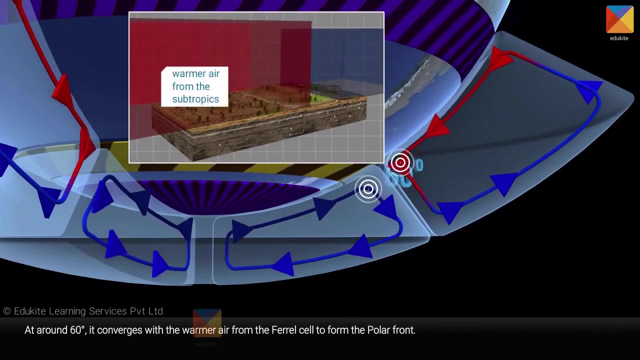 Low temperatures at the poles cause the air to subside At the surface. this subsiding air diverges and flows towards the equator as a surface wind. These are the polar easterlies. At around 60 degrees it converges with the warmer air from the ferrule cell to form the 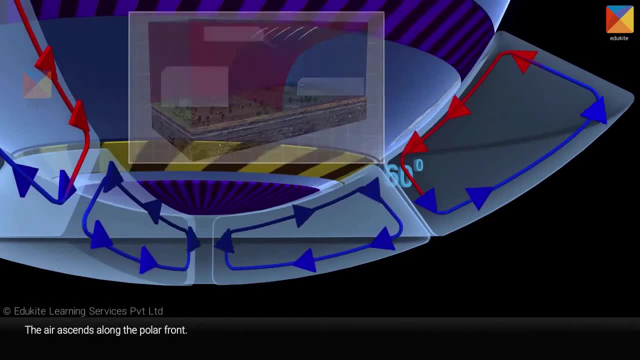 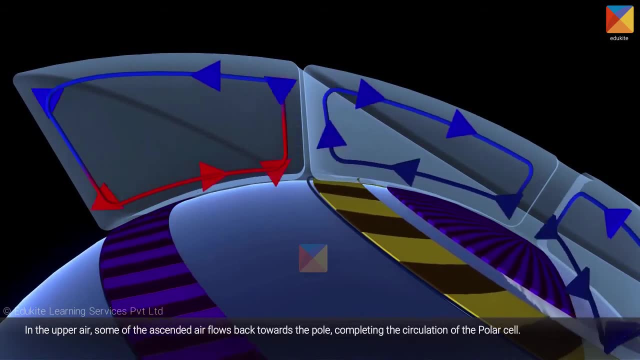 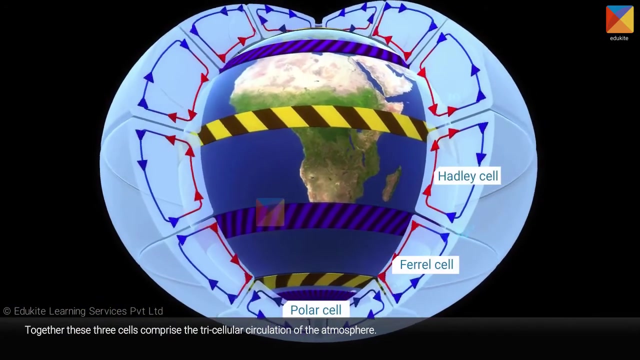 polar front. The air ascends along the polar front In the upper air. some of the ascended air flows back towards the pole, completing the circulation of the polar cell. Together, these three cells comprise the tricellular circulation of the atmosphere.